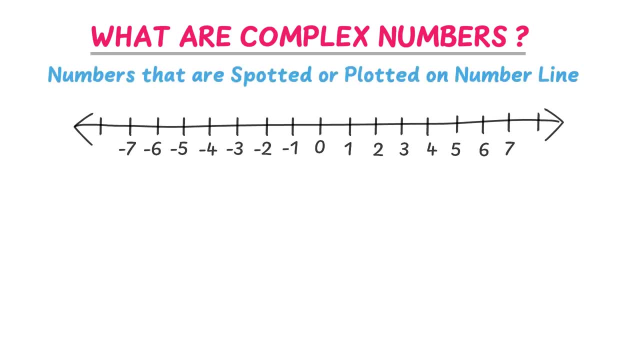 that all those numbers which can be spotted or plotted on a number line are real numbers, For example 3, minus 3, 4 and 6, etc. Now let's pick up any real number from the number line, For instance 4.. I add 4 plus 3i. 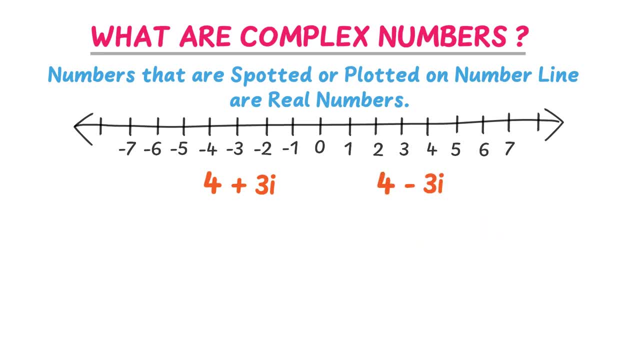 And then I subtract 4 minus 3i. Can you add or subtract these two numbers? Well, your answer would be: it is not possible to add or subtract real numbers like 4 and imaginary numbers like 3i, So we call it a complex number. We know that 4 is a real number. 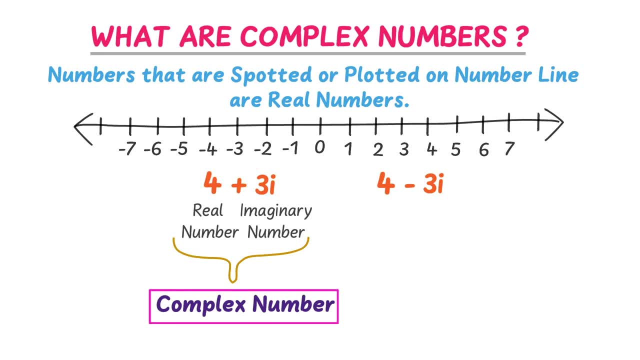 and 3i is an imaginary number, So complex numbers are made out of a real part and a point and imaginary part. Some other examples of complex numbers are 5 plus 6i, 3 minus 2i, 11 plus 2i, etc. Remember that the general form of complex numbers are a plus bi, where 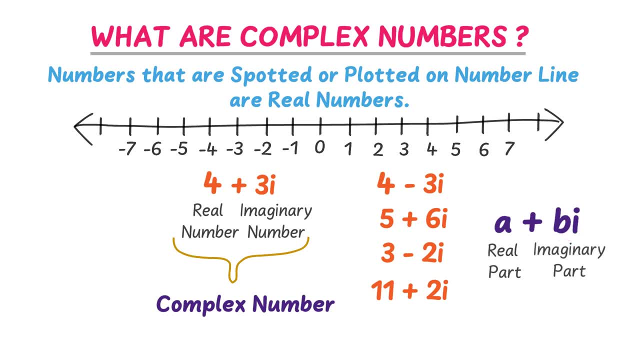 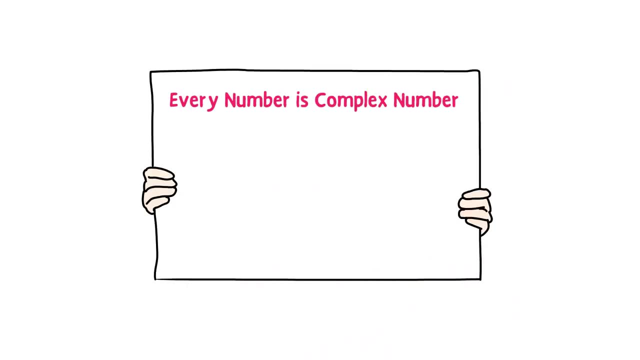 a is the real part and bi is the imaginary part. Finally, let me teach you a bonus concept. Remember that every number is complex number with zero as its imaginary part. Finally, let me teach you a bonus concept. Remember that every number is complex number with zero as its imaginary part. 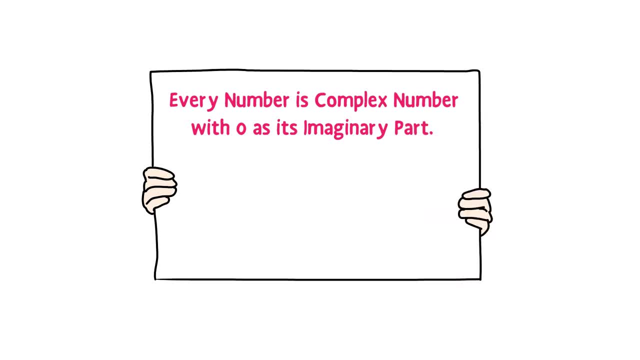 imaginary part. Let me repeat it: Every number is a complex number with zero as its imaginary part. For example, consider 7.. It is a real number. Now add 0i to the 7 as imaginary part. Note it down that 0 into iota is equal to 0. So 7 plus 0 is equal to 7.. We do not change. 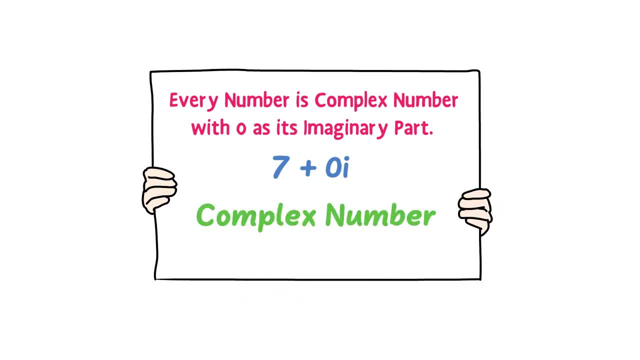 the value of 7.. So it becomes a complex number because of its real part and imaginary part. Therefore, we say that every real number is also considered as a complex number with zero as its imaginary part. Also, we learn that in our daily life we can make a simple